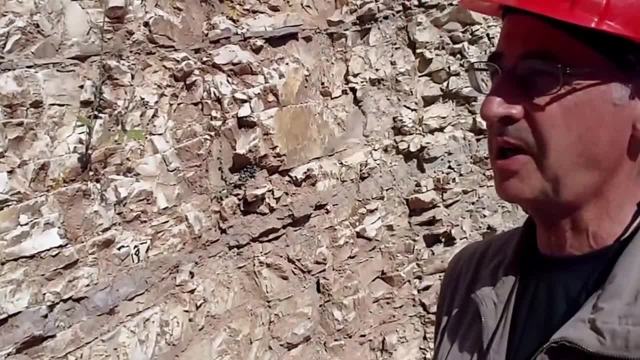 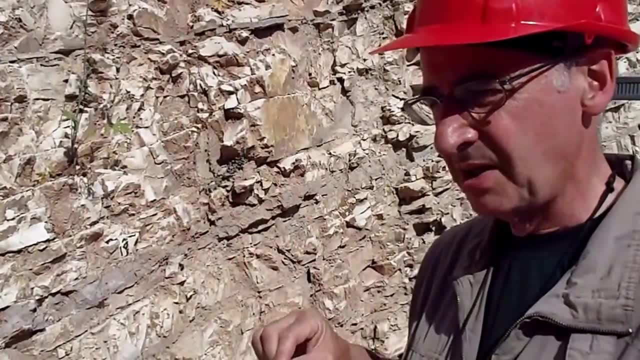 were apparently exactly the same age as the beds that you can see cropping out here in Italy, and of very high quality, Very, very similar character. So the idea was then that there was some global event which was very dramatic, which affected the whole of the ocean. 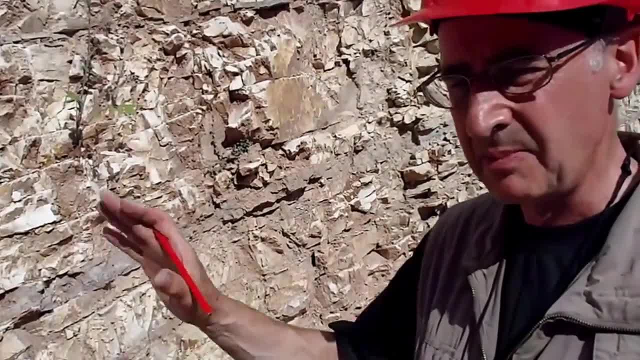 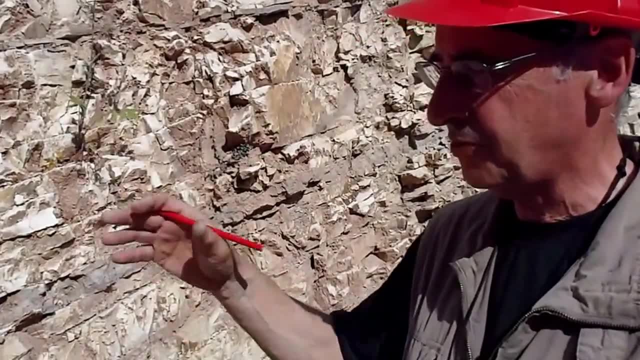 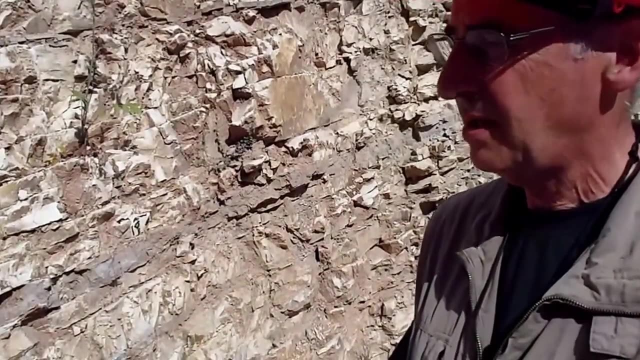 which allowed the accumulation of organic matter in many parts of the globe at the same time. In terms of time, we're talking about 93 million years ago. In terms of duration of that event, we're talking about maybe 200 to 300,, maybe 400,000 years. 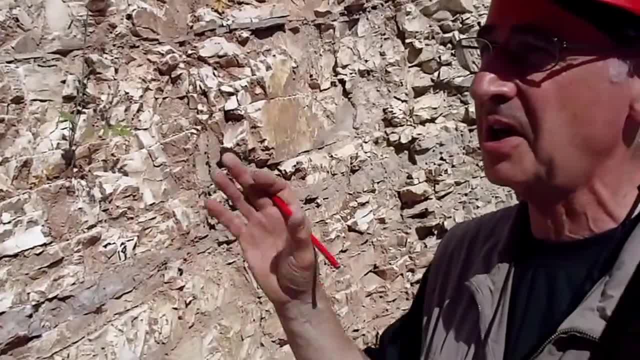 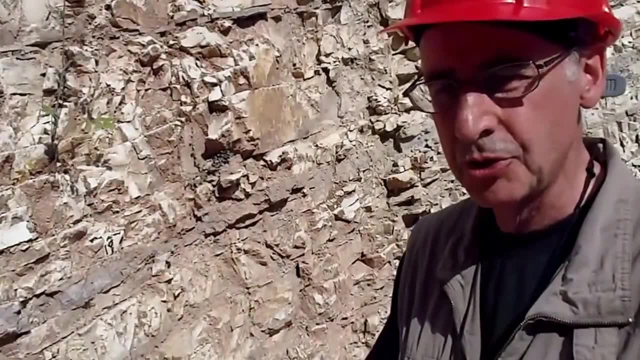 So that's the duration of the event. So that's the duration of the oceanic anoxic event. So the idea came from, really the insight that we gained from how the whole oceans work, from drilling in the middle of the Pacific Ocean. 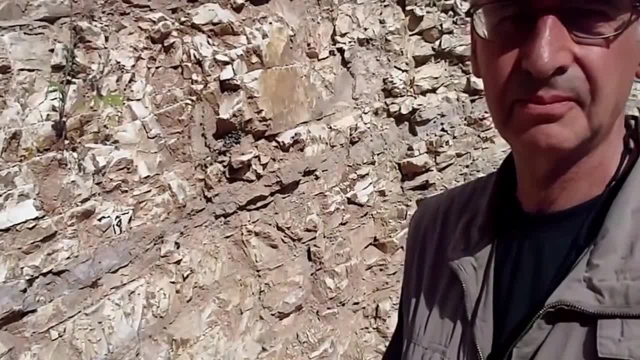 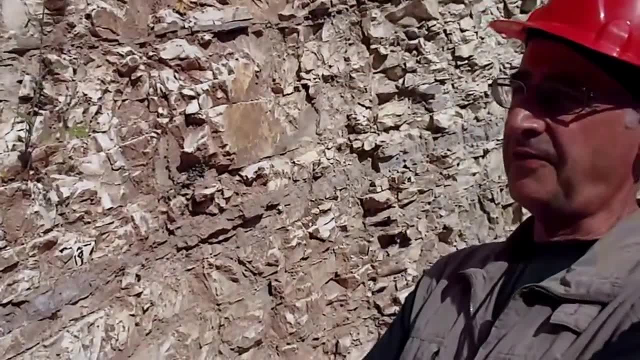 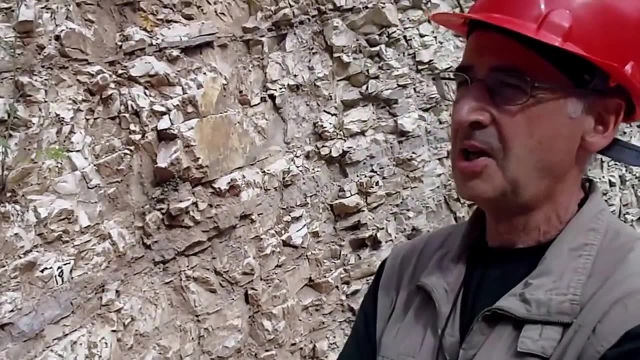 half a world away from right here in Italy. Why do you think that the oceanic anoxic events are important today? Well, for several reasons. If you're interested in petroleum source rocks, then that's exactly what they are. So if you have a feeling that petroleum source rocks were, 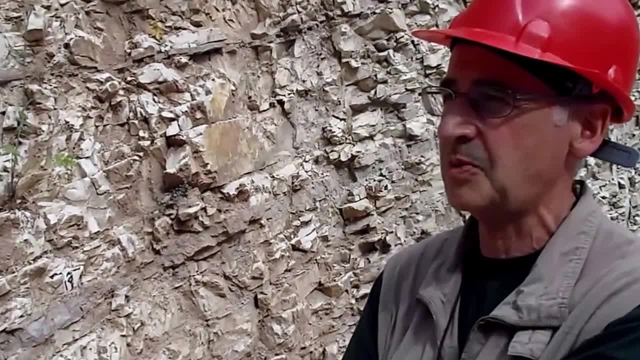 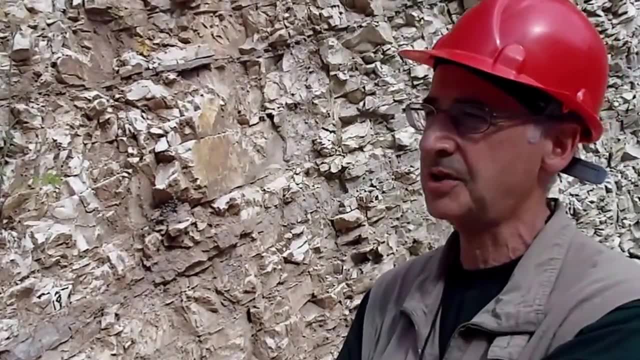 formed at certain instances in time. that could be something that could help in your exploration activities. They also give us a warning, perhaps, of what happens to the planet if you push it to very extreme conditions, And these oceanic anoxic events seem to have happened when the world was unusually warm. 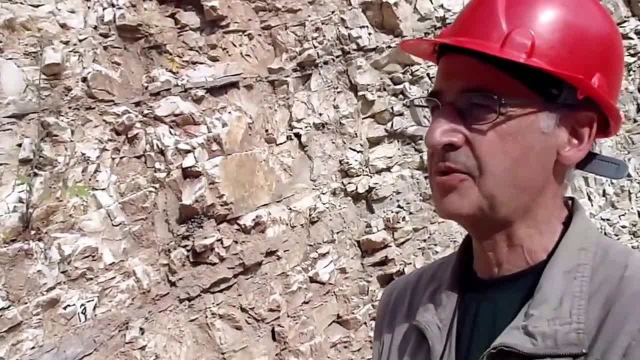 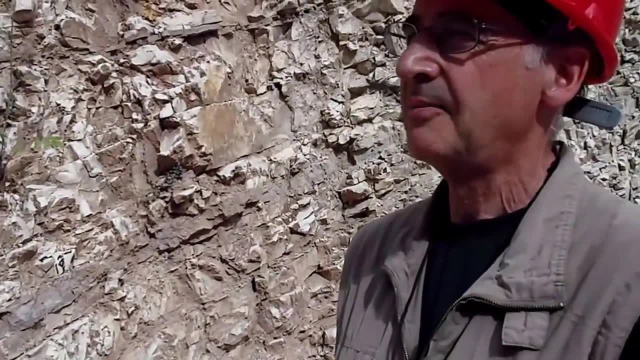 Warm because there were large amounts of carbon dioxide in the atmosphere. In this case, that probably came from huge volcanic eruptions in various parts of the globe during this interval of the year. During this interval of the year, During this interval of the year. 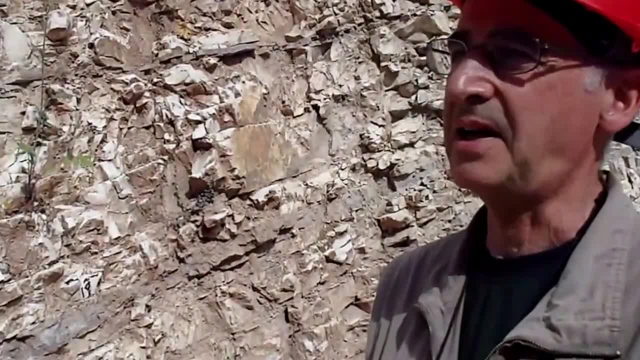 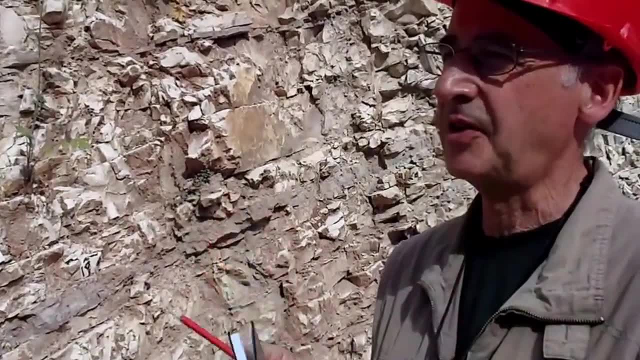 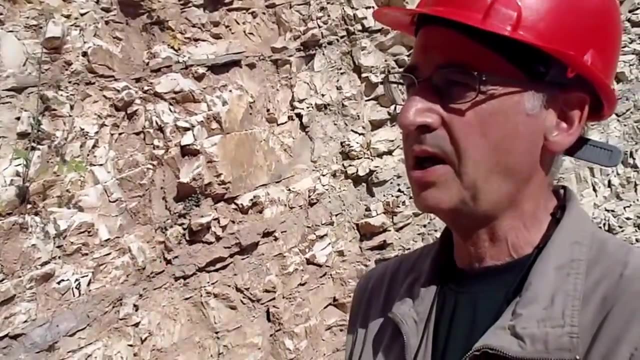 But if you want to take a lesson from what's happening to the planet now, we know it's warming, We know that certain conditions are changing in the oceans And some of the phenomena that we know characterize oceanic anoxic events are actually starting to happen in a very small way in the ocean today. 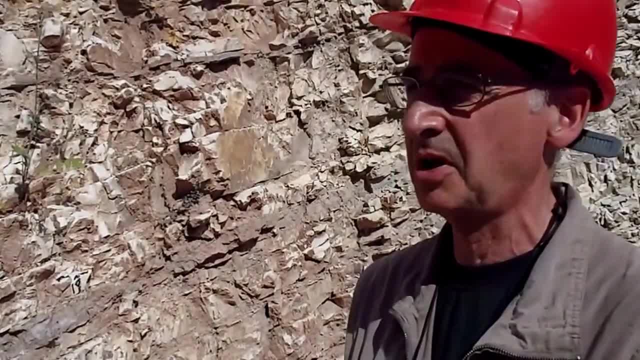 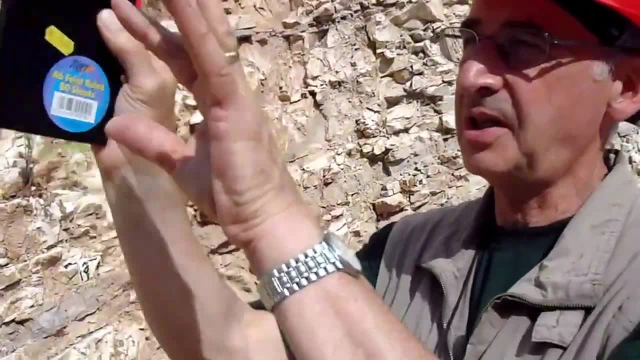 And that includes acidification of the oceans from the carbon dioxide but also spreading deoxygenation. So we don't know how this will evolve in future, but the, the geological sort of record here, tells you what happens if you push the planet very far.